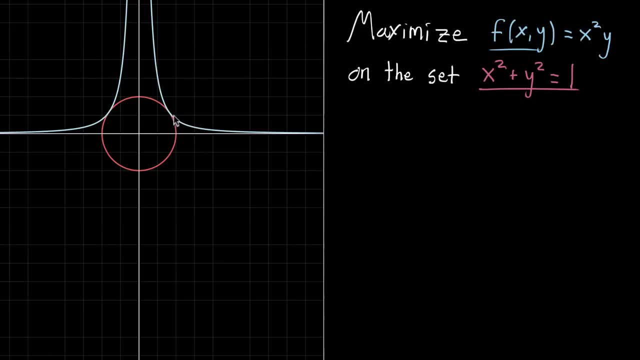 way we were visualizing this was to look at the xy plane, where this circle here represents our constraint. all of the points that make up this set, x squared plus y squared, equals one, And then this curvy line here is one of the contours of f, meaning we're setting. 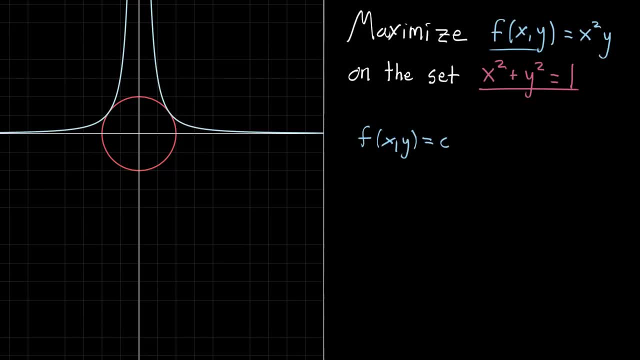 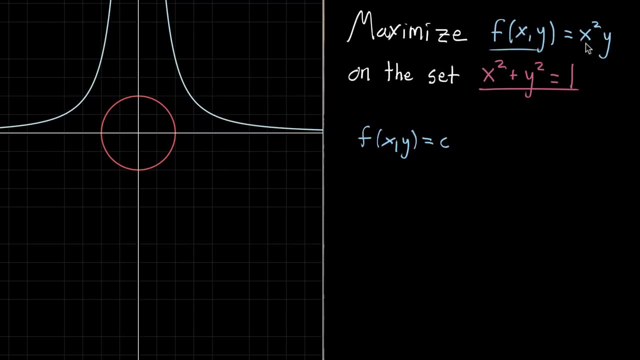 f of xy equal to some constant, and then I was varying around that constant c. So for high values of c, the contour would look something like this: This is where the value of x squared times y is big. And then for small values of c, the contours would look like this: So: 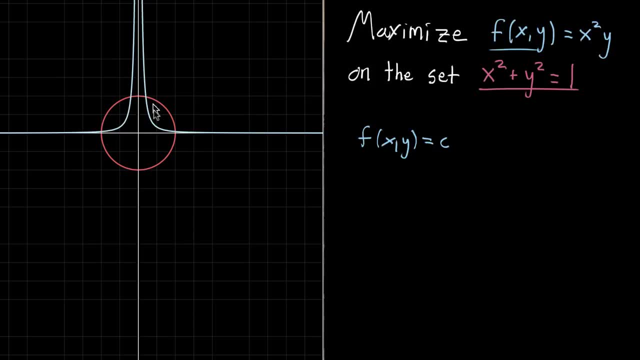 all the points on this line would be: f of xy equals like 0.01, in this case something like that. And the way to think about maximizing this function is to try to increase that value of c as much as you can without it falling off the circle. And the key observation is: 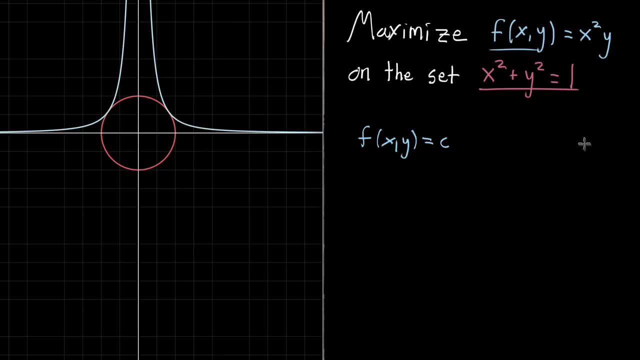 that happens when they're tangent. So you know, you might kind of draw this out in a little sketch and say: there's some curve representing your constraint, which in this case would be kind of where our circle is, And then the curve representing the contour would just 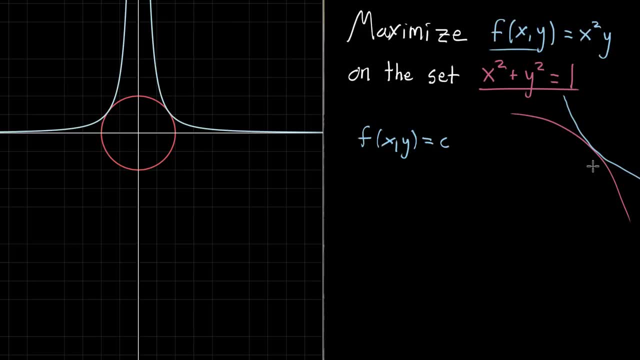 kiss that curve, just barely touch it in some way. Now that's pretty, but in terms of solving the problem, we still have some work to do, And the main tool we're going to use here is the gradient. So let me go. 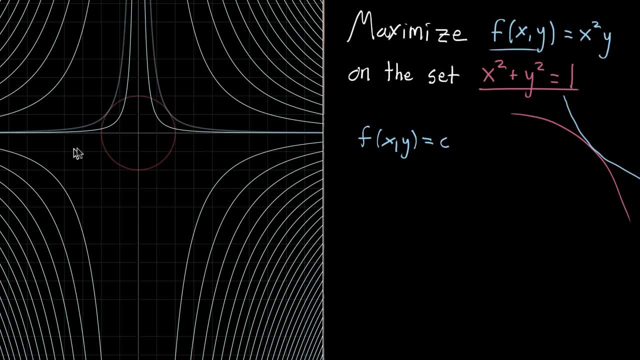 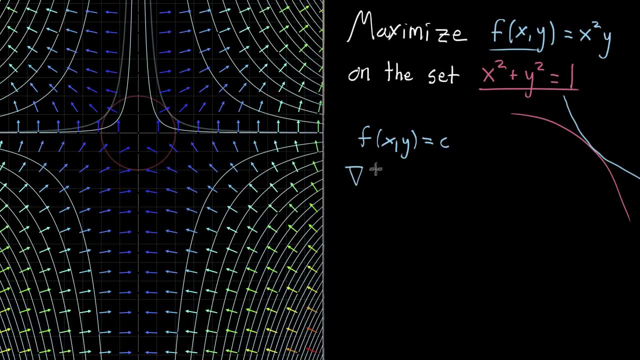 ahead and draw a lot more contour lines than there already are for x squared times y. So this is many of the contour lines And I'll draw the gradient field, the gradient field of f. So I've made a video about the relationship between the gradient and contour lines And 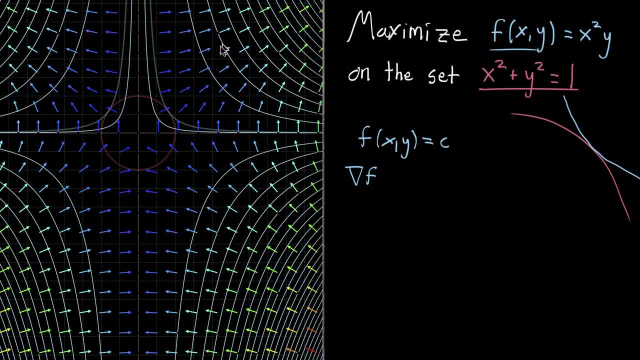 the upshot of it is that these gradient vectors, every time they pass through a contour line, they're perpendicular to it, And the basic reason for that is if you walk along the contour line, the function isn't changing value. So if you want it to change, 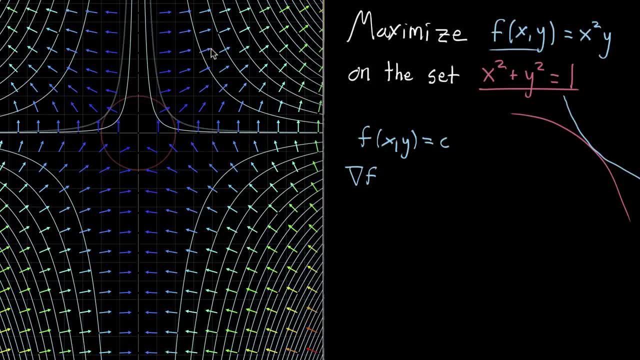 most rapidly. you know it kind of makes sense you should walk in the perpendicular direction so that no component of the walk that you're taking is, you know, useless, is along the line where the function doesn't change. But again, there's a whole video on that, that's. 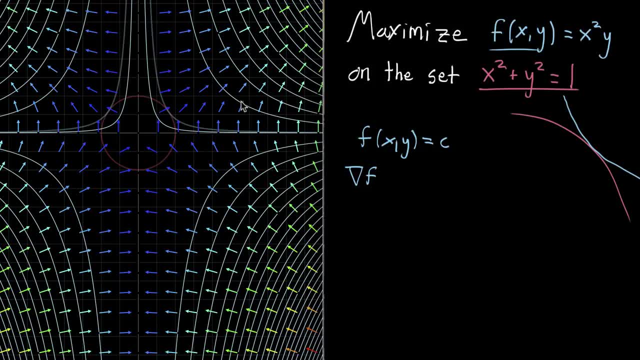 worth checking out if this feels unfamiliar For our purposes. what it means is that when we're considering this point of tangency, the gradient of f at that point is going to be some vector Perpendicular to both of the curves at that point, So that little vector represents the 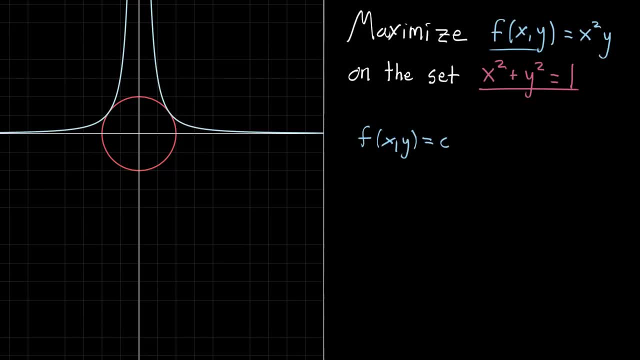 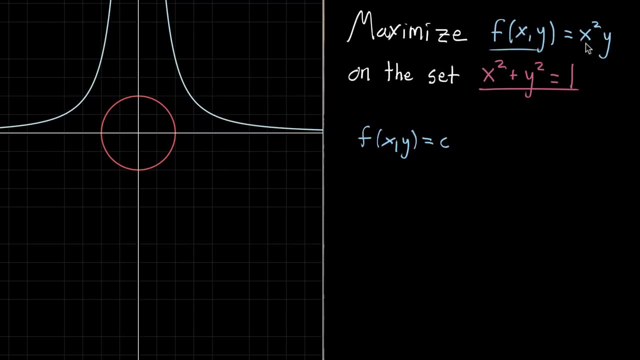 f of xy equal to some constant, and then I was varying around that constant c. So for high values of c, the contour would look something like this: This is where the value of x squared times y is big. And then for small values of c, the contours would look like this: So: 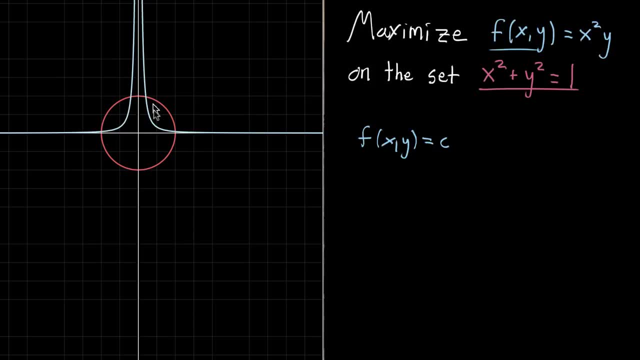 all the points on this line would be: f of xy equals like 0.01, in this case something like that. And the way to think about maximizing this function is to try to increase that value of c as much as you can without it falling off the circle. And the key observation is: 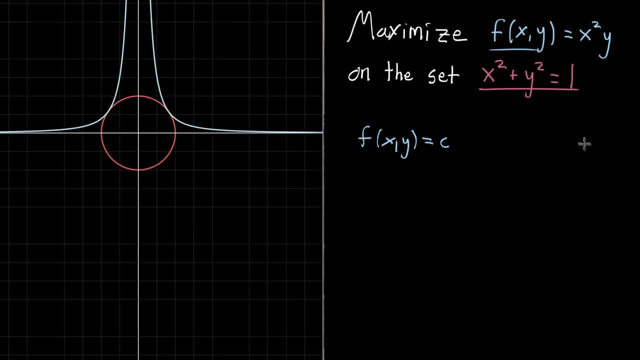 that happens when they're tangent. So you know, you might kind of draw this out in a little sketch and say there's some curve representing your constraint, which in this case would be, you know kind of, where our circle is, And then the curve representing the contour. 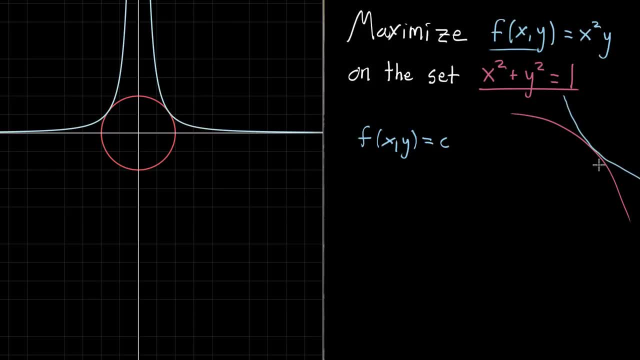 would just kiss that curve, just barely touch it in some way. Now that's pretty, but in terms of solving the problem, we still have some work to do, And the main tool we're going to use here is the gradient. So let me go. 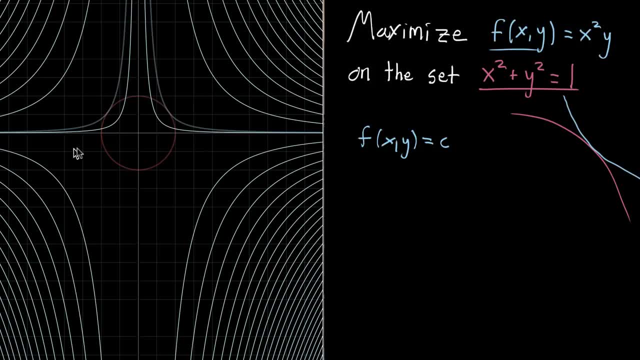 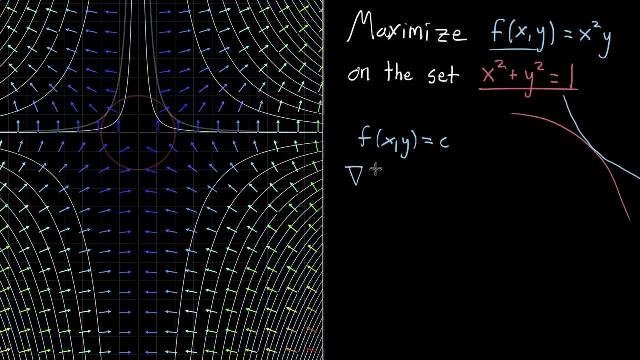 ahead and draw a lot more contour lines than there already are for x squared times y. So this is many of the contour lines And I'll draw the gradient field, the gradient field of f. So I've made a video about the relationship between the gradient and contour lines And 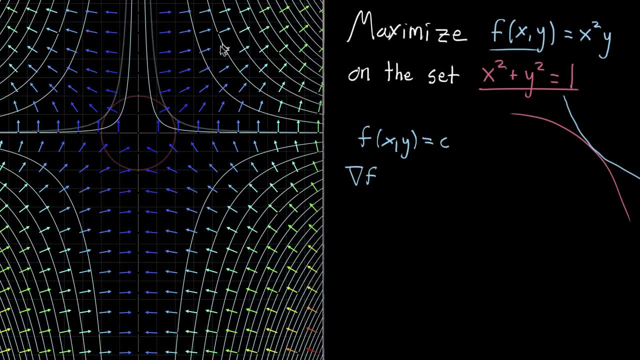 the upshot of it is that these gradient vectors, every time they pass through a contour line, they're perpendicular to it, And the basic reason for that is if you walk along the contour line, the function isn't changing value. So if you want it to change, 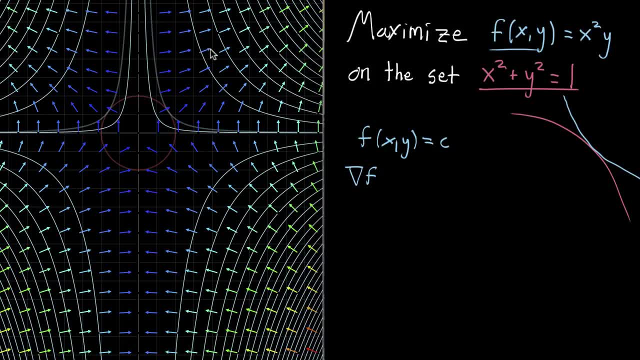 most rapidly. you know it kind of makes sense you should walk in the perpendicular direction so that no component of the walk that you're taking is, you know, useless, is along the line where the function doesn't change. But again, there's a whole video on that, that's. 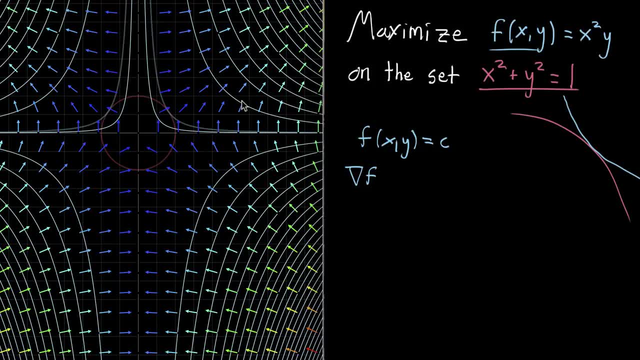 worth checking out if this feels unfamiliar For our purposes. what it means is that when we're considering this point of tangency, the gradient of f at that point is going to be some vector. It's going to be perpendicular to both of the curves at that point. So that little vector. 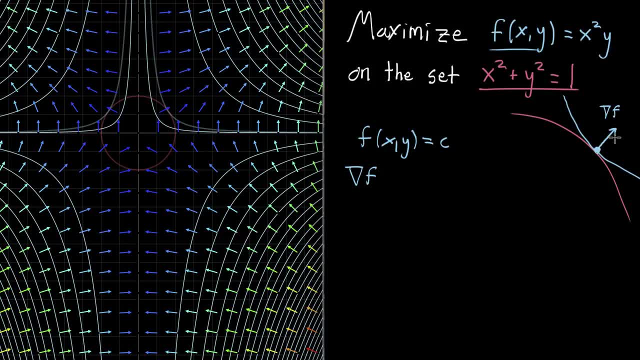 represents the gradient of f at this point on the plane, And we can do something very similar to understand the other curve Right now. I've just written it as a constraint: x squared plus y squared equals one. But you know, to give that function a name, let's 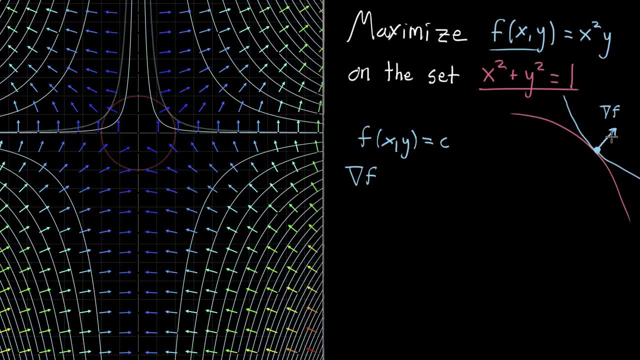 gradient of f at this point on the plane And we can do something very similar to understand the other curve Right now. I've just written it as a constraint: x squared plus y squared equals one, But you know to give that function. 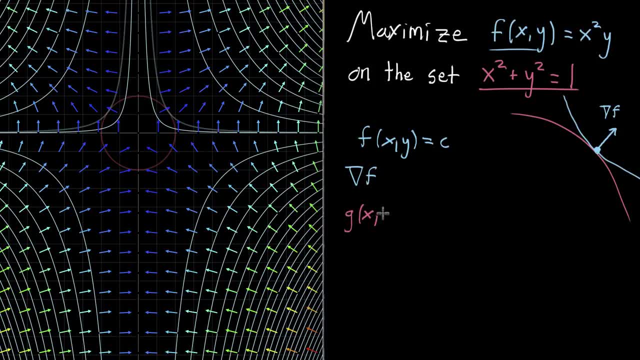 a name. let's say that we've defined g of xy to be x squared plus y squared, x squared plus y squared. In that case, this constraint is pretty much just one of the contours that are drawn in relation to the contact lines of the function g, And we could take a look. 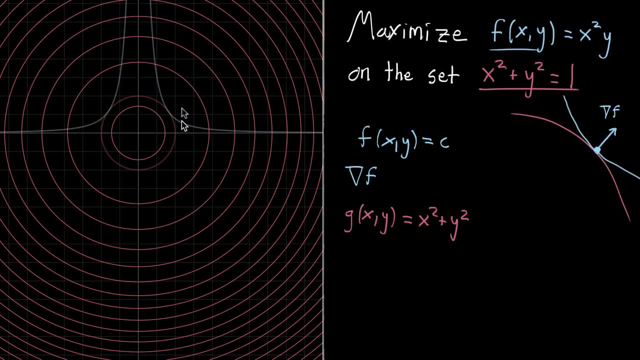 at that. And if we go over here and we look at all of the other contour lines for this function g- and it should make sense that they're circles because this function is x squared plus y squared- And if we took a look at the gradient of g, if we go over and ask 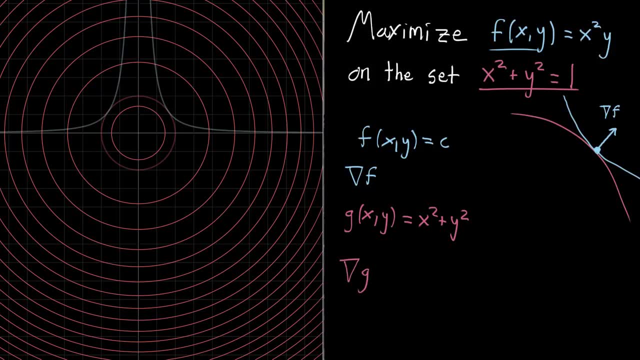 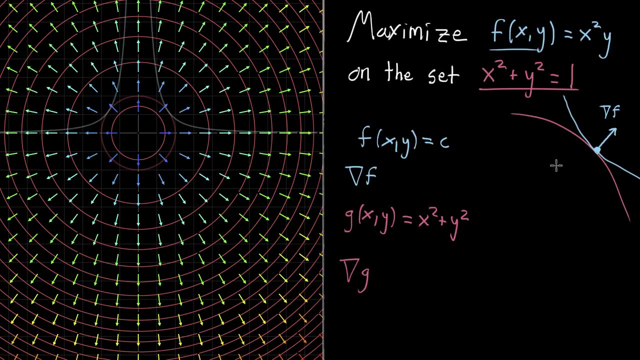 about the gradient of g. it has that same property That every gradient vector, if it passes through a contour line, is perpendicular to it. So over on our drawing here, the gradient vector of g has a line to the other side of the contours, And what's so weird about thisUM? 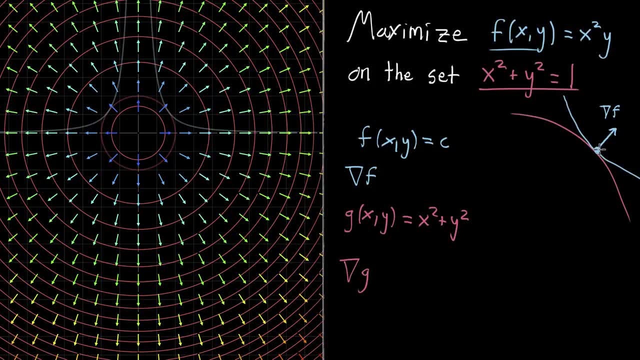 It has a line to the other side of the contours, But every time you've taken that line, you're would also be perpendicular to both these curves. And you know, maybe in this case it's not as long as the gradient of f, or maybe it's longer. 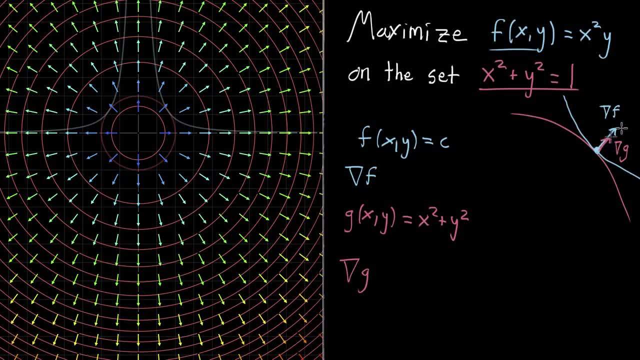 There's no reason that it would be the same length, but the important fact is that it's proportional, And the way that we're gonna write this in formulas is to say that the gradient of f, evaluated- let's see evaluated at whatever the maximizing value. 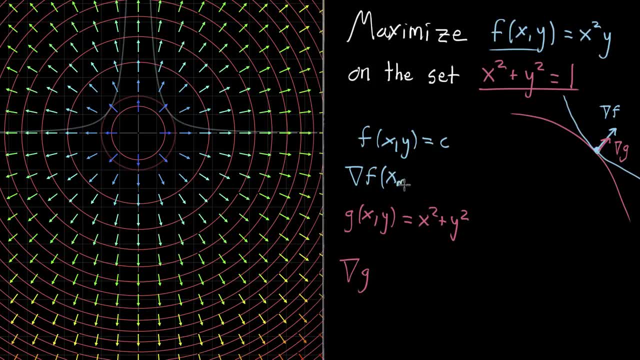 of x and y are, so we should give that a name- probably Maybe x sub m, y sub m, The specific values of x and y that are gonna be at this point. that maximizes the function subject to our constraint. So that's gonna be related to the gradient of g. 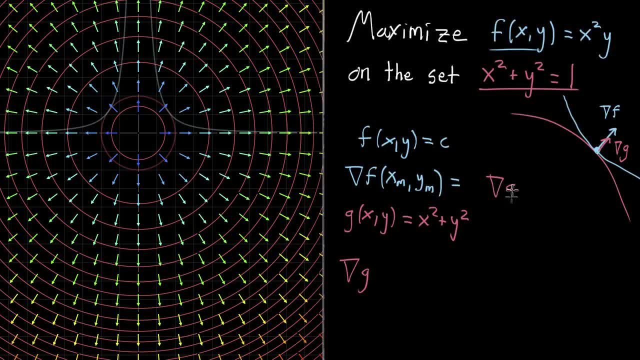 It's not gonna be quite equal, so I'll leave some room here Related to the gradient of g evaluated at that same point. xm, ym, And, like I said, they're not equal, they're proportional. So we need to have some kind of 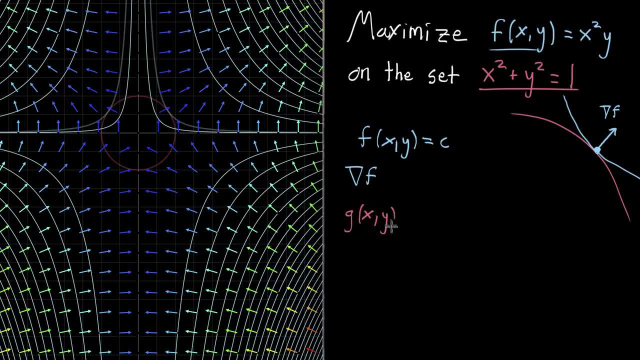 say that we've defined g of xy to be x squared plus y squared, x squared plus y squared. In that case this constraint is pretty much just one of the contour lines for the function g, And we can take a look at that If we go over 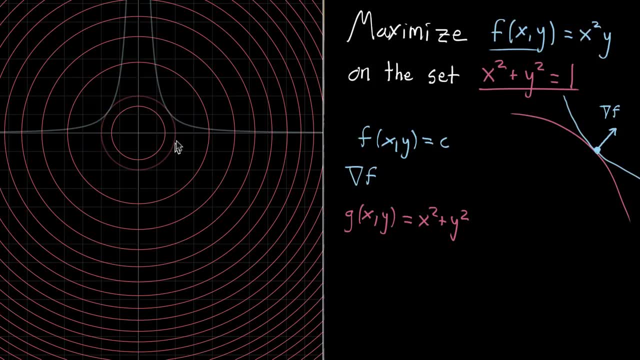 here and we look at all the other contour lines for this function g, and it should make sense that they're circles, because this function is x squared plus y squared. And if we took a look at the gradient of g and we go over and ask about the gradient of g, 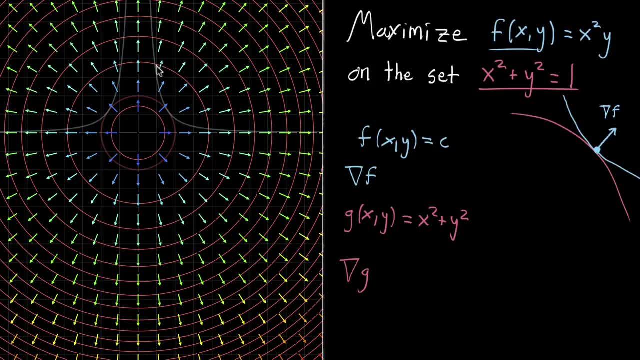 it has that same property, That every gradient vector, if it passes through a contour line, is perpendicular to it. So over on our drawing here, vector of g would also be perpendicular to both these curves. And you know, maybe in this case it's not as long. 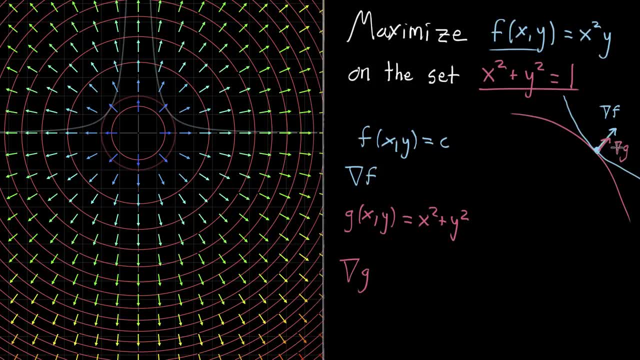 as the gradient of f, or maybe it's longer. there's no reason that it would be the same length, but the important fact is that it's proportional, And the way that we're gonna write this in formulas is to say that the gradient of f, evaluated. 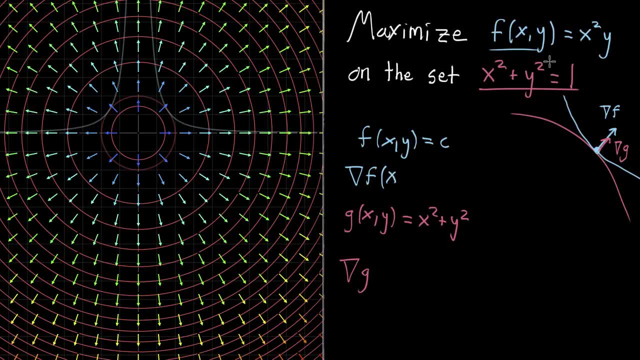 let's see, evaluated at whatever the maximizing value of x and y are. so we should give that a name: probably maybe x sub m, y sub m, the specific values of x and y that are gonna be at this point. that maximizes. 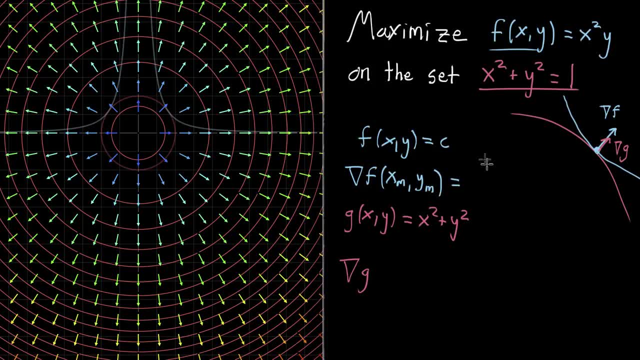 the function subject to our constraint. So that's gonna be related to the gradient of g. it's not gonna be quite equal, so I'll leave some room here related to the gradient of g evaluated at that same point. xm ym. 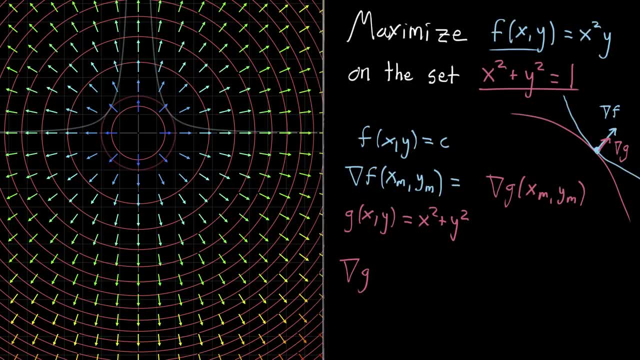 And, like I said, they're not equal, they're proportional. so we need to have some kind of proportionality constant in there, and you almost always use the variable lambda, and this guy has a fancy name: it's called a Lagrange multiplier. 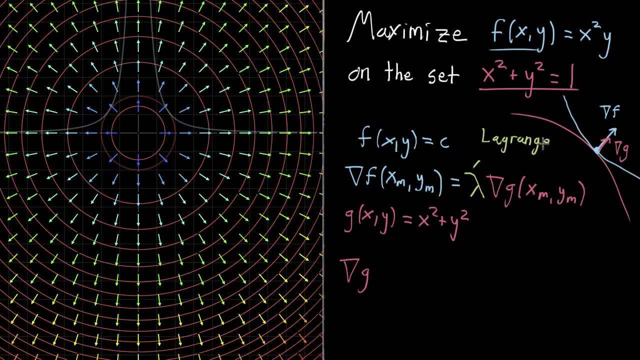 Lagrange. Lagrange was one of those famous French mathematicians. I always get him confused with some of the other French mathematicians at the time, like Legendre or Laplace. there's a whole bunch of things. Let's see multiplier. distracting myself talking here. 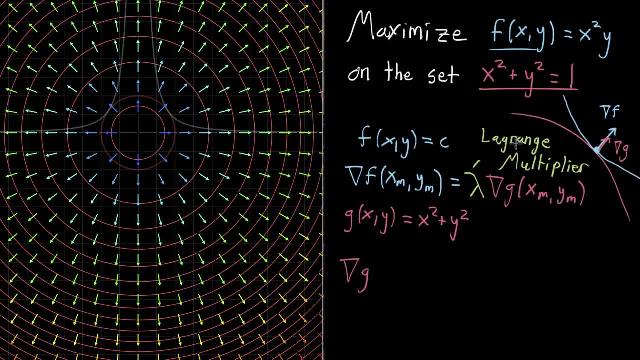 So Lagrange multiplier, So there's a number of things in multivariable calculus named after Lagrange, and this is one of the big ones. This is a technique that he kind of developed or at the very least popularized, and the core idea. 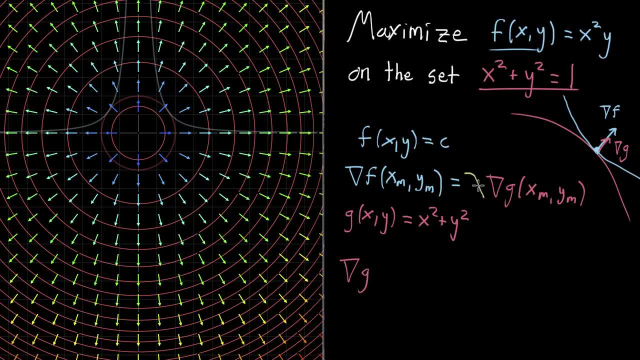 proportionality constant. in there You almost always use the variable lambda. and this guy has a fancy name: It's called a Lagrange multiplier. Lagrange was one of those famous French mathematicians. I always get him confused with some of the other. 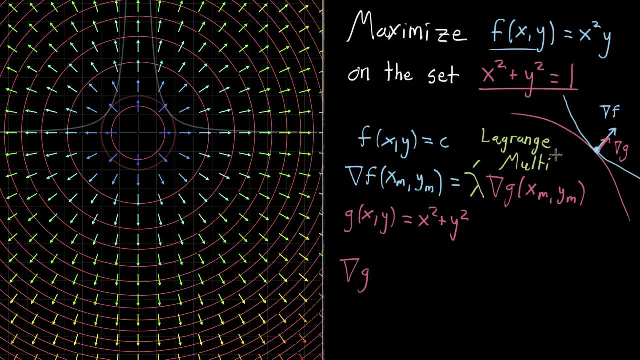 French mathematicians at the time, like Legendre or Laplace. There's a whole bunch of things. Let's see multiplier, distracting myself talking here. So Lagrange, multiplier, So there's a number of things in multivariable calculus named after Lagrange and this is one of the big ones. 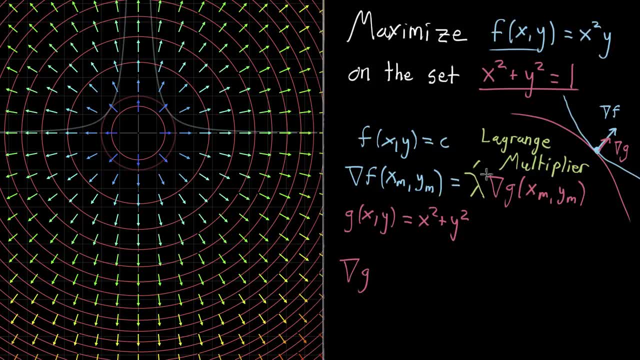 This is a technique that he kind of developed, or at the very least popularized, and the core idea is to just set these gradients equal to each other, because that represents when the contour line for one function is tangent to the contour line of another. 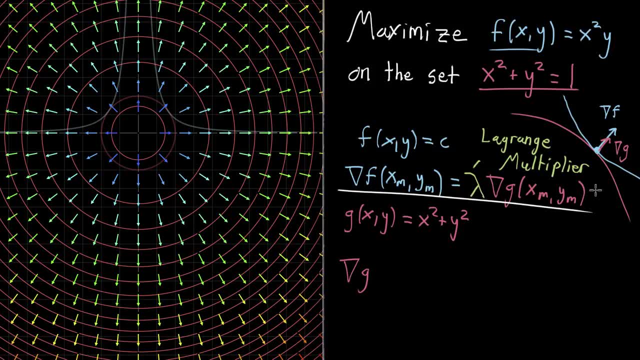 So this, this is something that we can actually work with, And let's start working it out right. Let's see what this translates to in formulas. So I already have g written here, so let's go ahead and just evaluate what the gradient of g should be. 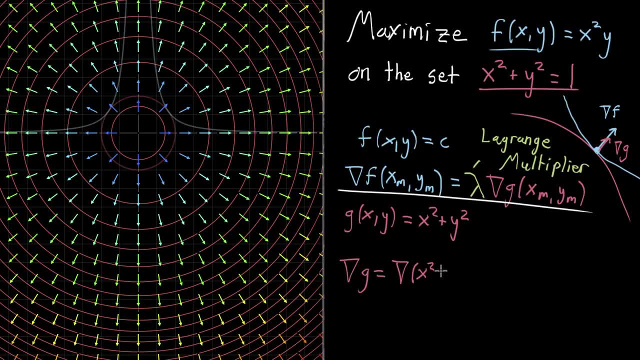 And that's the gradient of x squared plus y squared. And the way that we take our gradient is it's gonna be a vector whose components are all the partial derivatives. So the first component is the partial derivative with respect to x. so we treat x as a variable. 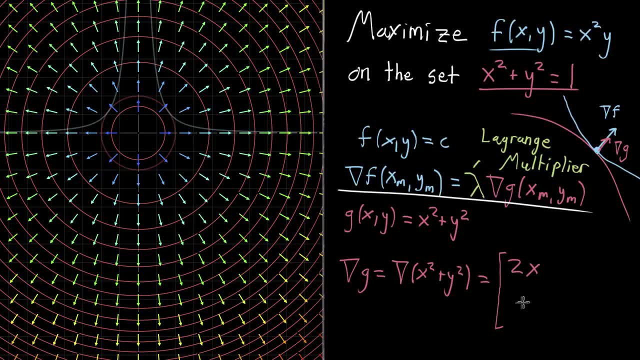 y looks like a constant. the derivative is two x. The second component, the partial derivative with respect to y. so now we're treating y as the variable, x as the constant, so the derivative looks like two y. Okay, so that's the gradient of g. 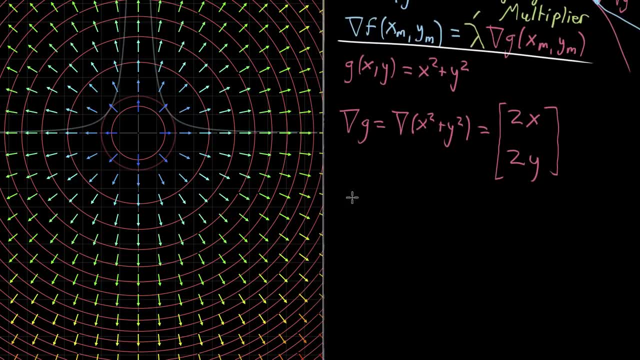 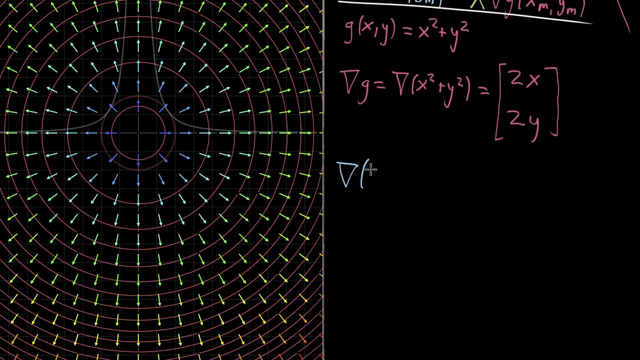 And then the gradient of f. gradient of f, it's gonna look like gradient of. let's see what is x, What is f. It's x squared times y. So x squared times y, we do the same thing. First component, partial derivative, with respect to x. 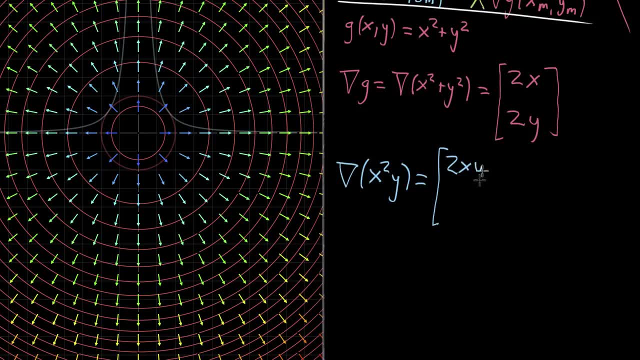 x looks like a variable, so its derivative is two times x, and then that y looks like a constant when we're up here, But then partial derivative with respect to y, that y looks like a variable, that x, squared, just looks like a constant sitting in front of it. 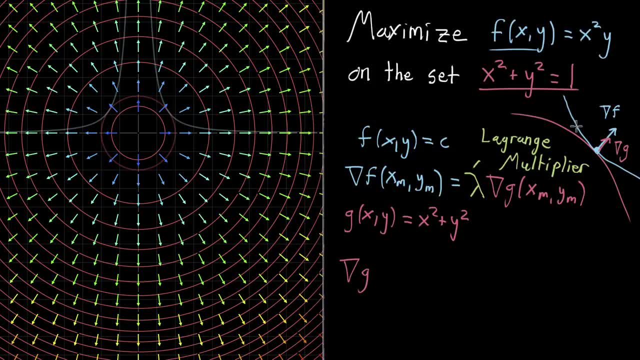 is to just set these gradients equal to each other, because that represents when the contour line for one function is tangent to the contour line of another. So this, this, is something that we can actually work with, And let's start working it out right. 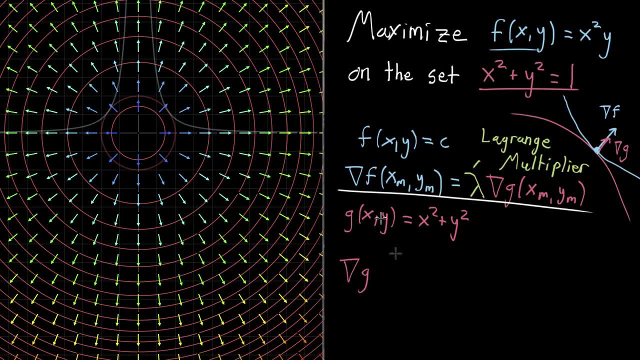 Let's see what this translates to in formulas. So I already have g written here, so let's go ahead and just evaluate what the gradient of g should be, And that's the gradient of x squared plus y squared And the way that we take our gradient. 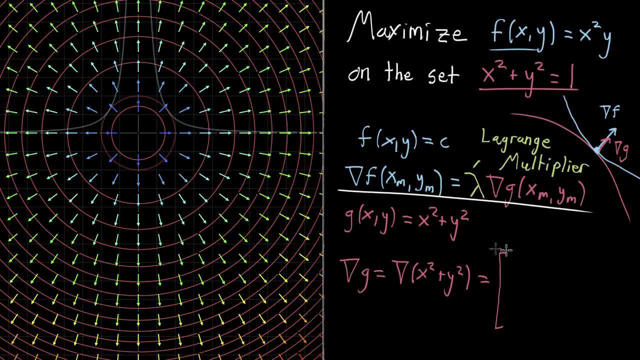 is. it's going to be a vector whose components are all the partial derivatives. So the first component is the partial derivative with respect to x. so we treat x as a variable. y looks like a constant. the derivative is 2x. The second component, the partial derivative. 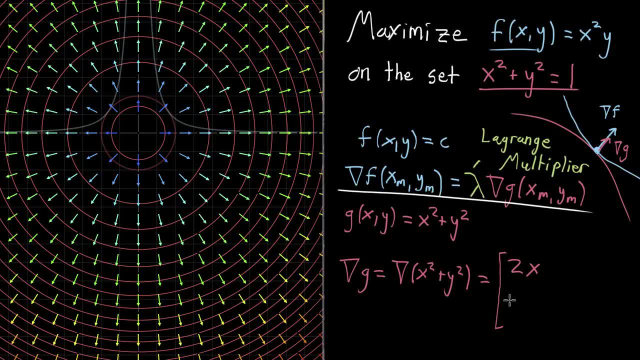 with respect to y. so now we're treating y as the variable, x as the constant. so the derivative looks like 2y. Okay, so that's the gradient of g And then the gradient of f. gradient of f is going to look like: 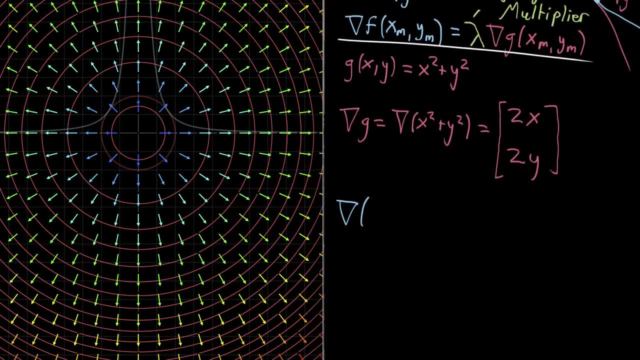 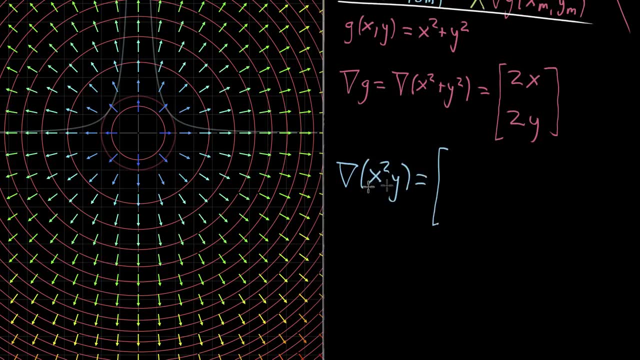 let's see what is x, What is f? It's x squared times y, So x squared times y. we do the same thing. First component: partial derivative. with respect to x. x looks like a variable, so its derivative is 2x. 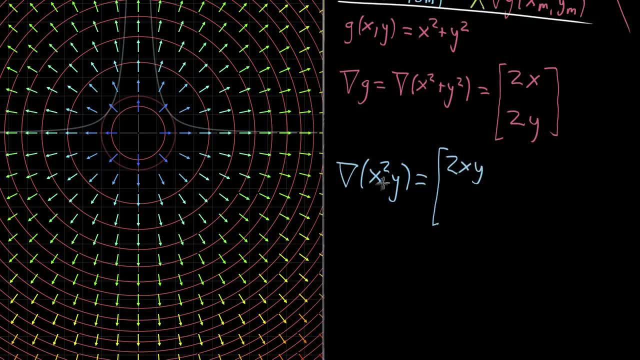 and then that y looks like a constant when we're up here, But then, partial derivative with respect to y, that y looks like a variable, that x, squared, just looks like a constant sitting in front of it. So that's what we get. 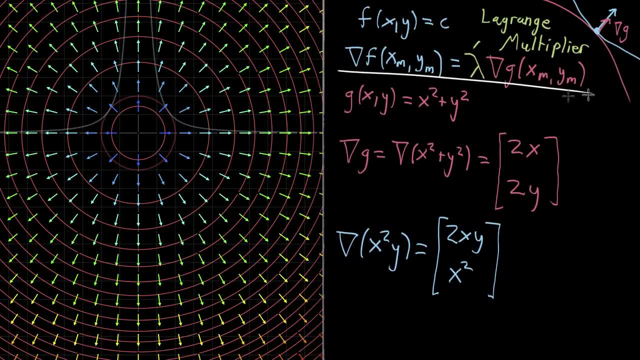 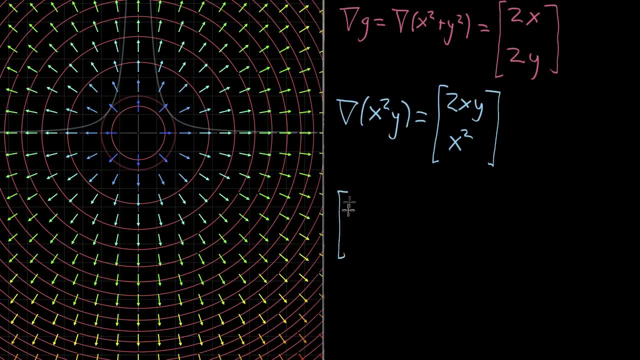 And now, if we kind of work out this Lagrange multiplier expression using these two vectors, what we have written, what we're going to have written, is that this vector, 2xy x squared, is proportional, with a proportionality constant lambda, to the gradient vector for g. 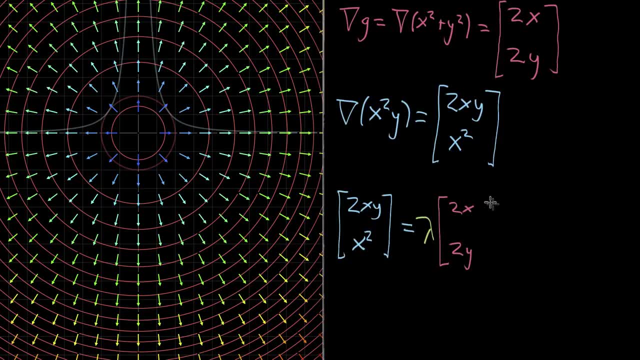 to 2x, 2y And, if you want, you can think about this as two separate equations. I mean, right now it's one equation with vectors, but really what this is saying is you've got two separate equations. 2 times xy is equal to lambda. 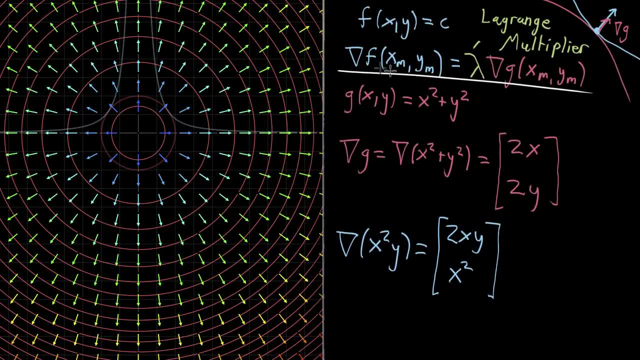 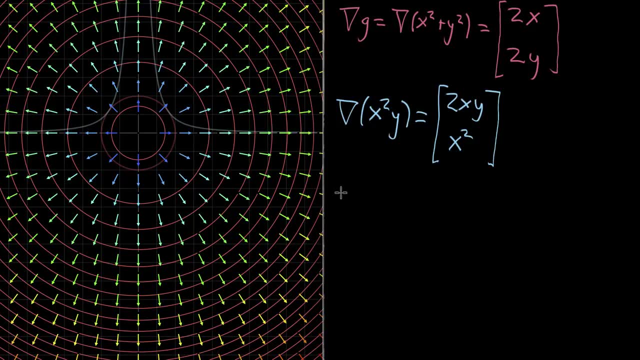 So that's what we get. And now, if we kind of work out this Lagrange multiplier expression using these two vectors, what we have written, what we're gonna have written, is that this vector two- x, y, x squared, is proportional with a proportionality constant lambda. 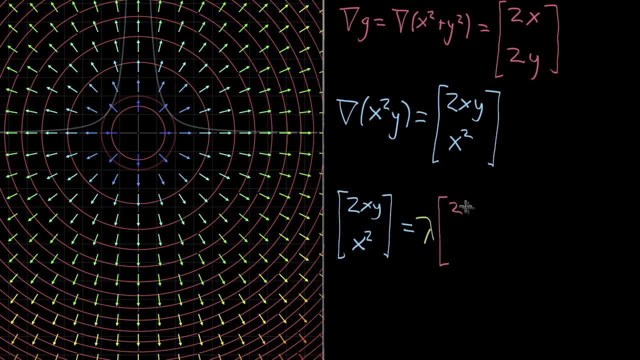 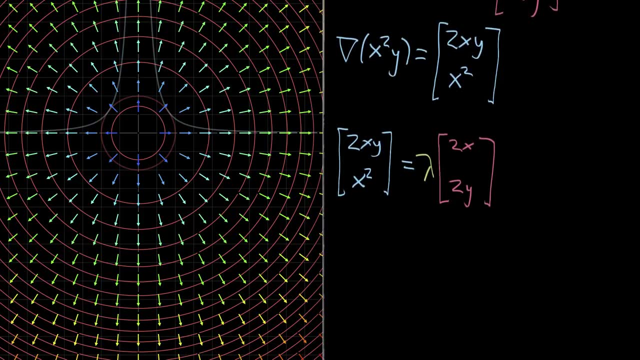 to the gradient vector for g to two x, two y And, if you want, you can think about this as two separate equations. I mean, right now it's one equation with vectors, but really what this is saying is: you know, you've got two separate equations. 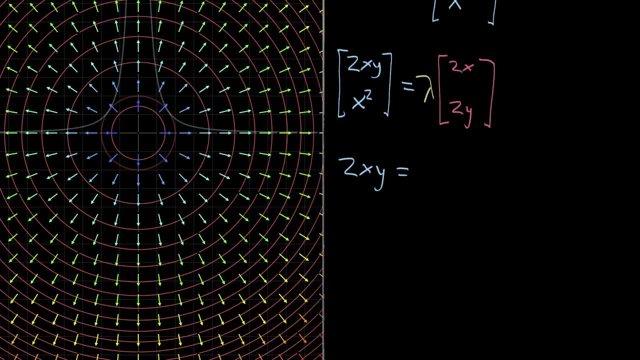 Two times x, y is equal to lambda. ah, gotta change colors a lot here. lambda times two x. hmm, gonna be a stickler for color. Keep red all of the things associated with g. And then the second equation is that x squared. 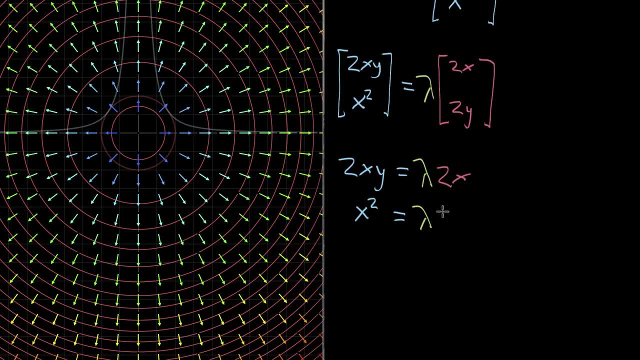 is equal to lambda times two y, And this might seem like a problem because we have three unknowns: x, y and this new lambda that we introduced, kind of shot ourselves in the foot by giving ourselves a new variable to deal with. But we only have two equations. 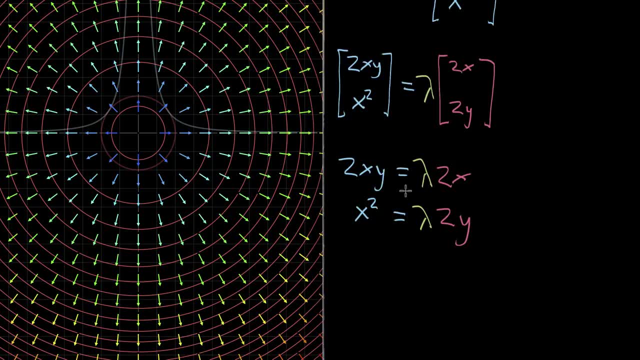 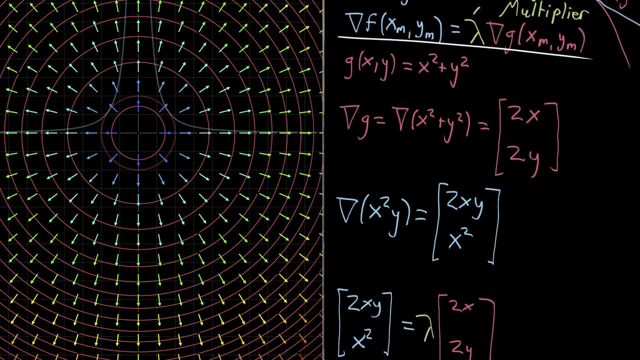 So, in order to solve this, we're gonna need three equations, And the third equation is something that we've known the whole time. It's been part of the original problem. It's the constraint itself: x squared plus y, x squared plus y squared- excuse me- equals one. 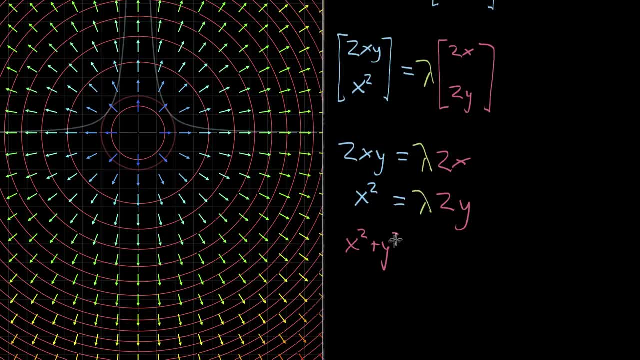 So that that third equation, x squared plus y squared, Y squared is equal to one. So these are the three equations that characterize our constrained optimization problem. The bottom one just tells you that we have to be on this unit circle here. 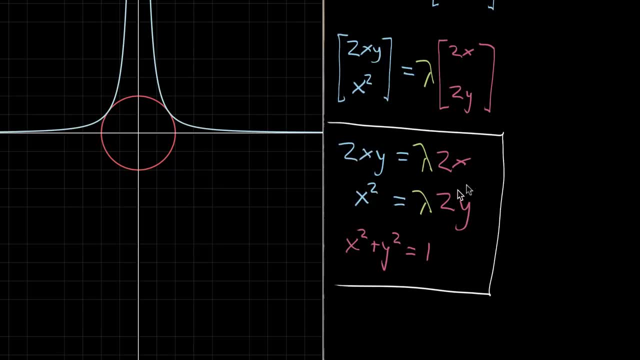 Let me just highlight it: We have to be on this unit circle, And then these top two tell us what's necessary in order for our contour lines, the contour of F and the contour of G, to be perfectly tangent with each other. So in the next video I'll go ahead and solve this. 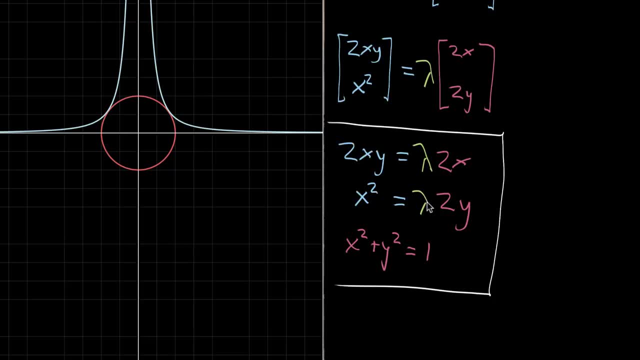 At this point it's pretty much just algebra to deal with, but it's worth going through. And then the next couple ones. I'll talk about a way that you can encapsulate all three of these equations into one expression, and also a little bit about the interpretation. 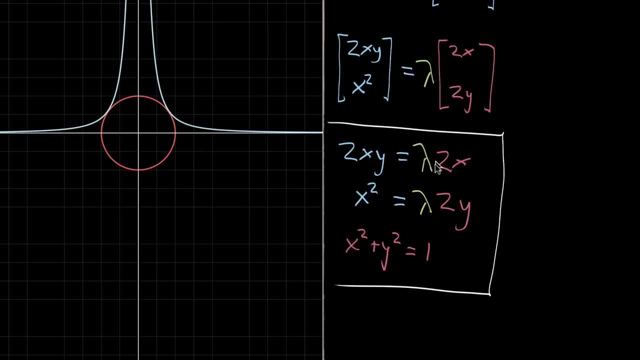 of this lambda that we introduced, Because it's not actually just a dummy variable. It has a pretty interesting meaning in physical context once you're actually dealing with a constrained optimization problem in practice. So I'll see you next video. 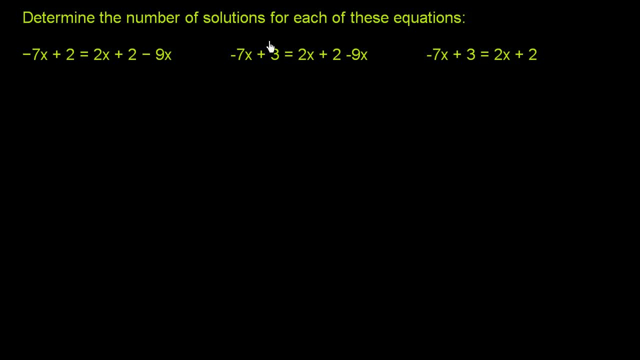 Determine the number of solutions for each of these equations, And they give us three equations right over here, And before I deal with these equations in particular, let's just remind ourselves about when we might have one or infinite or no solutions. You're going to have one solution if you can. 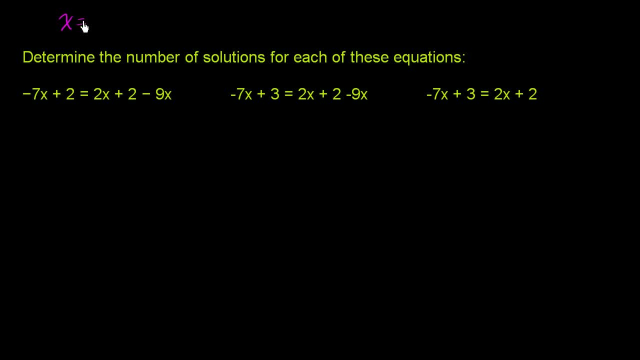 by solving the equation, come up with something like x is equal to some number. Let's say x is equal to. if I want to say in the abstract, x is equal to a, Or if we actually were to solve it, we get something like x equals 5 or 10 or negative pi. 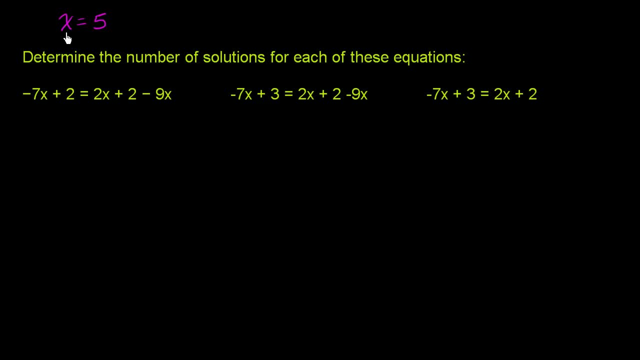 whatever it might be, But if you could actually solve for a specific x, then you have one solution. So this is one solution, just like that. Now, if you go and you try to manipulate these equations in completely legitimate ways, but you end up, 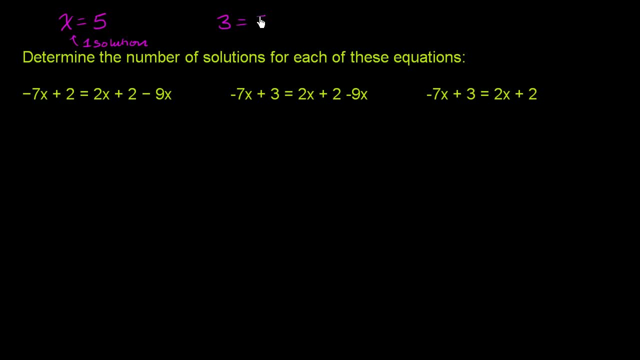 with something crazy like 3 equals 5,, then you have no solutions. And if you just think about it reasonably, all of these equations are about, well, finding an x that satisfies this. And if you were to just keep simplifying it? 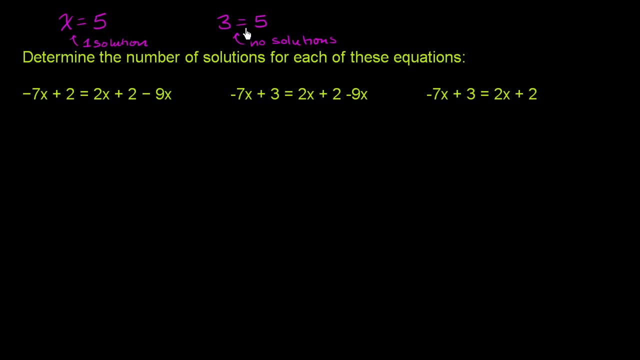 and you were to get something like 3 equals 5, and you were to ask yourself the question: is there any x that can somehow magically make 3 equal 5?? No, No x can magically make 3 equal 5.. So there's no way that you can make. 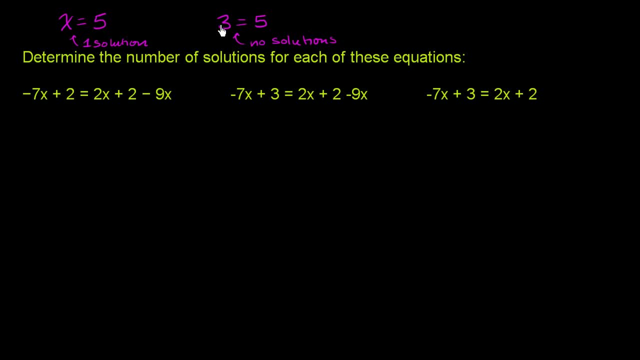 this thing be actually true, no matter which x you pick. So if you get something very strange like this, this means there's no solution. On the other hand, if you get something like, 5 equals 5, and I'm just overusing the number 5.. 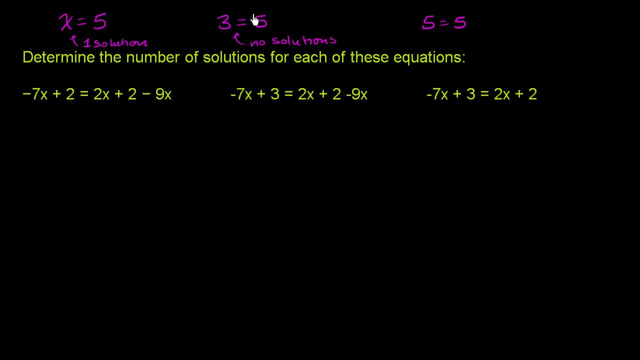 It didn't have to be the number 5.. It could be 7 or 10 or 113, whatever, And actually let me just not use 5, just to make sure that you don't think it's only for 5..